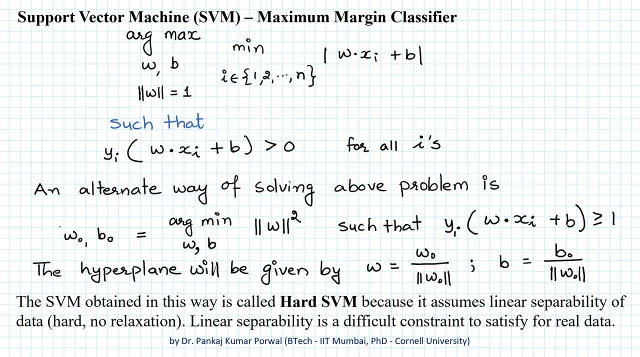 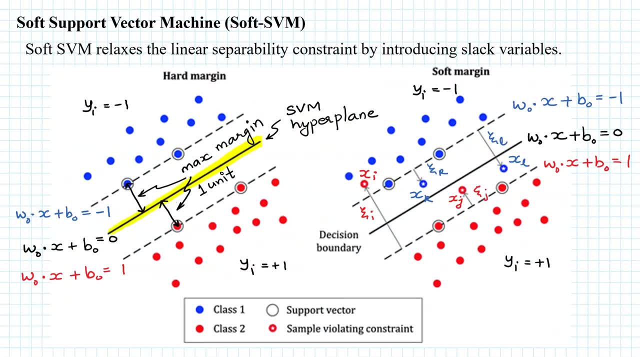 equation in alternate formulation of support vector machine. So in hard support vector machine algorithm we want the data to be not only linearly separable, but we want all the data points in both the classes, So for example here the blue class as well as the. 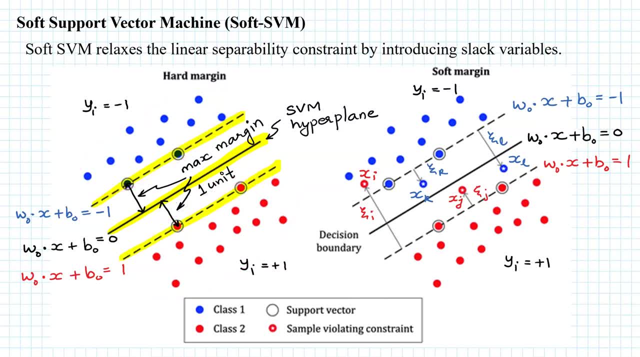 red class to be at least one unit distance away from our separating vector machine. So, �� So, we can use hard support vector machine algorithm to checks for this result so, in vector machine algorithm does is it relaxes this hard linear separability constraint by introducing slack variables and the slack variable measures 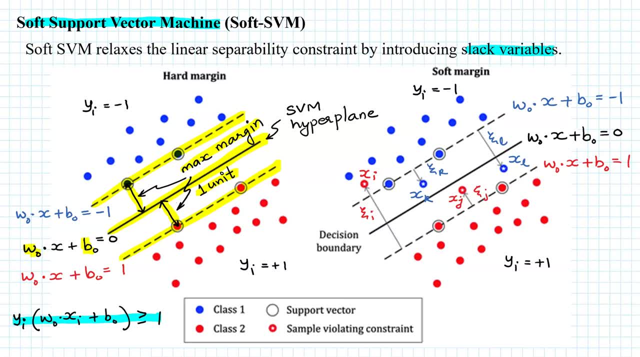 extent of violation of our linear separability constraint by individual data points. so here, for example, we see that these two blue data points and these two red data points violate our linear separability constraint and the slack variables. psi I's measure the extent of violation of linear 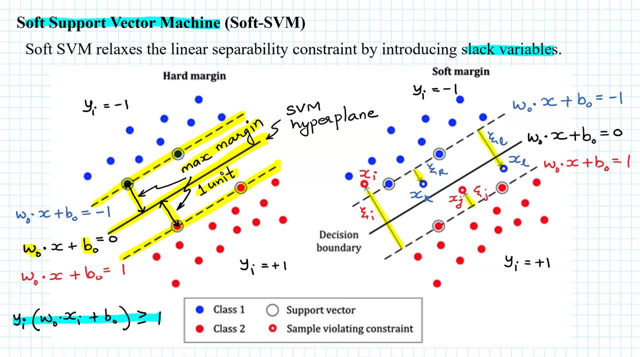 separability constraint for each of these data points. so, rather than value of product y i into w? naught, dot X i plus b? naught being greater than equals to one, it becomes y i 了什麼 into w0. dot xi plus b0 should be greater than equals to 1 minus xi i for point xi and this: 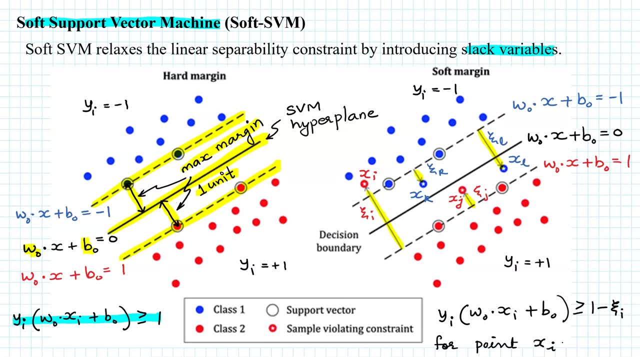 we modify for all the data points in our blue as well as red classes. So here we note that we expected all our data points to be at least one unit distance away from our separating hyperplane. but if a data point violates our constraint then it will be at a distance 1 minus xi i distance. 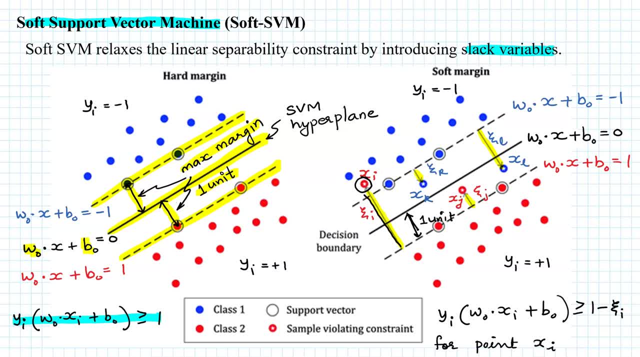 away from our separating hyperplane and you note that the violation of the constraint may be less than one unit, which is the case for the data point xk and xj, and it can also be more than one unit, which is the case for data point xi and xl, which